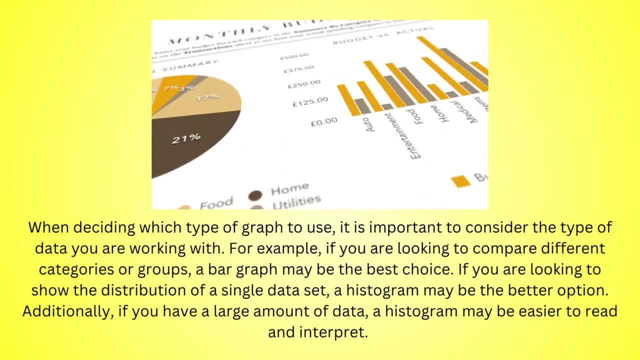 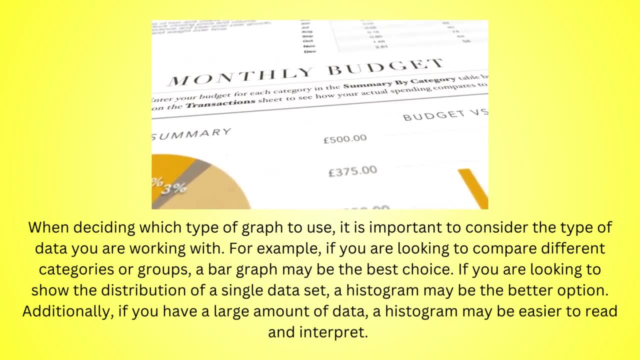 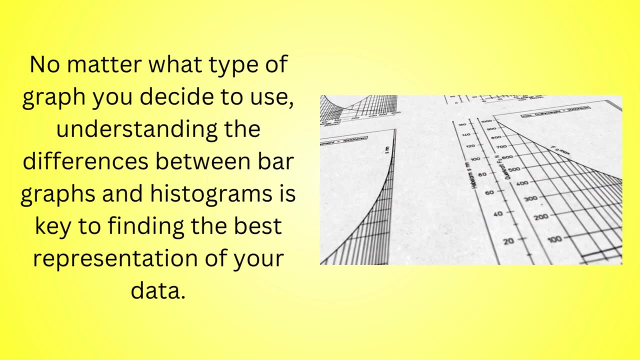 a single data set, a histogram may be the better option. Additionally, if you have a large amount of data, a histogram may be easier to read and interpret. No matter what type of data you are working with, you can use a histogram to show the distribution. 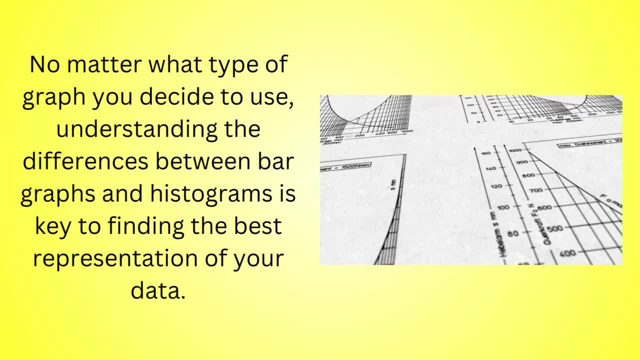 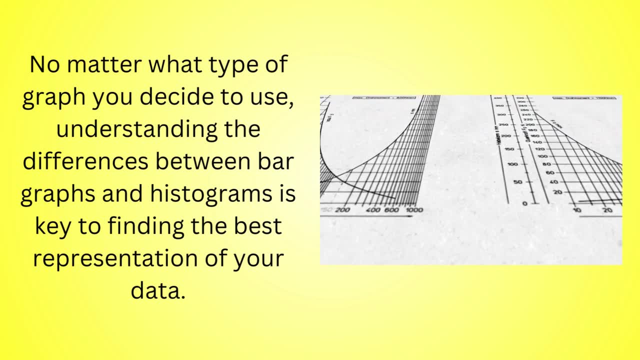 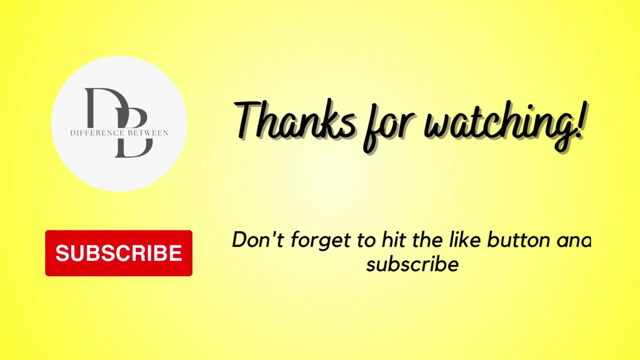 of a single data set. No matter what type of graph you decide to use, understanding the differences between bar graphs and histograms is key to finding the best representation of your data. Thanks for watching. Don't forget to hit the like button and subscribe. 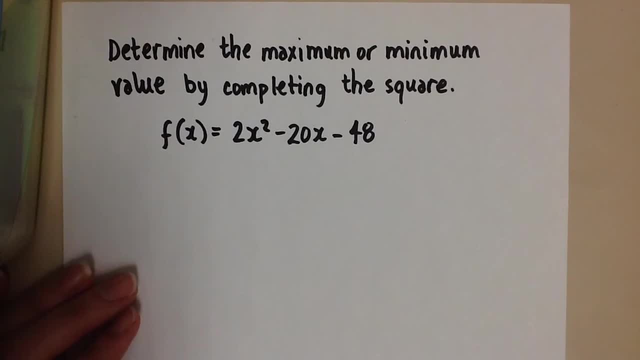 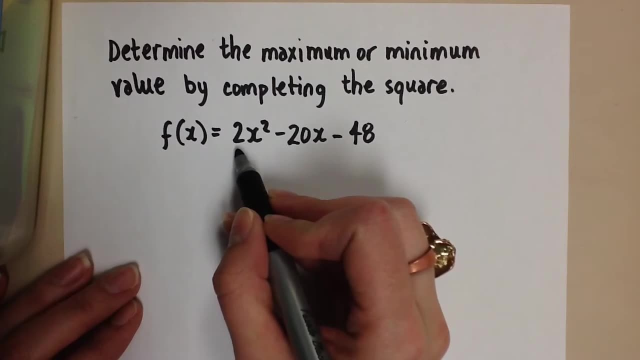 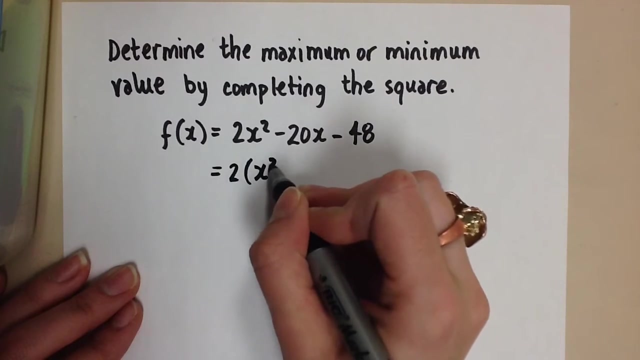 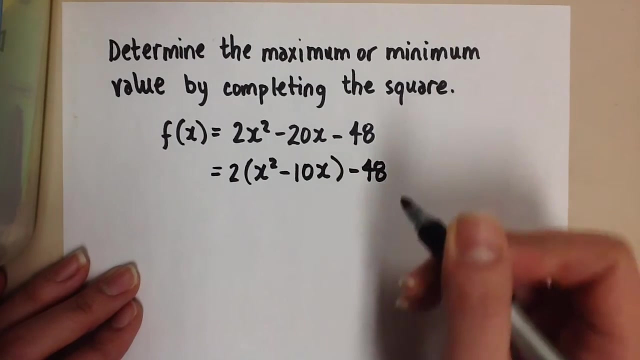 Here we're going to find the maximum or the minimum of this quadratic by completing the square. So to start, we see that the x squared term has a coefficient of 2. We want to factor that out of the first two terms only, So we get x squared minus 10x in the brackets and we leave that minus 48 outside of the brackets. 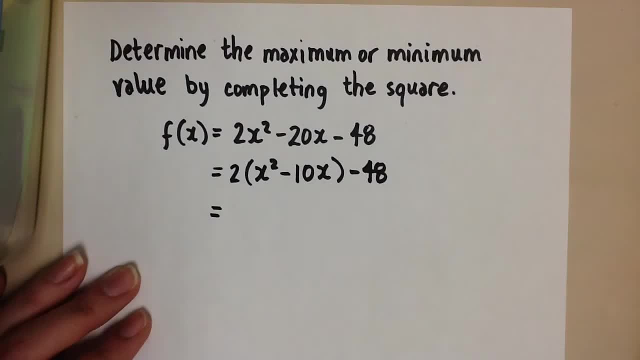 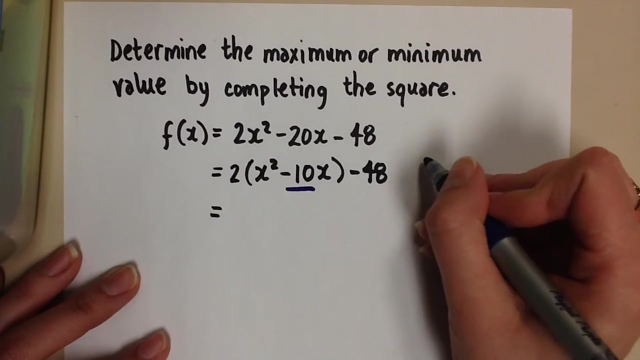 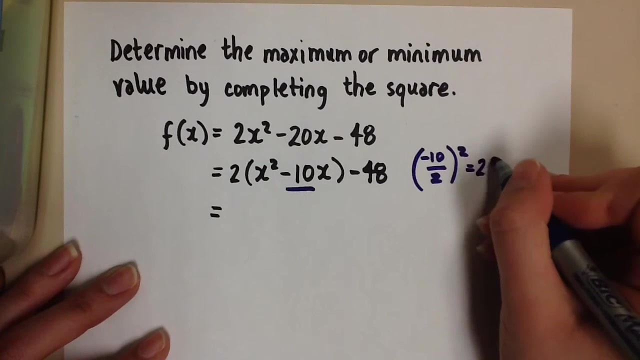 Then to find out what we're going to add and subtract from the equation in order to manipulate this into a perfect square, we're going to take that coefficient of the x term and divide it by 2, then square it. This gives us 25.. 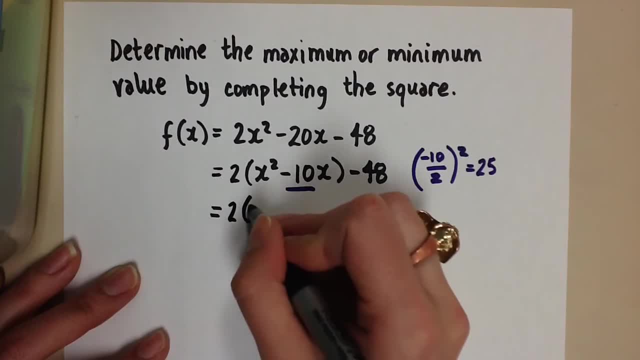 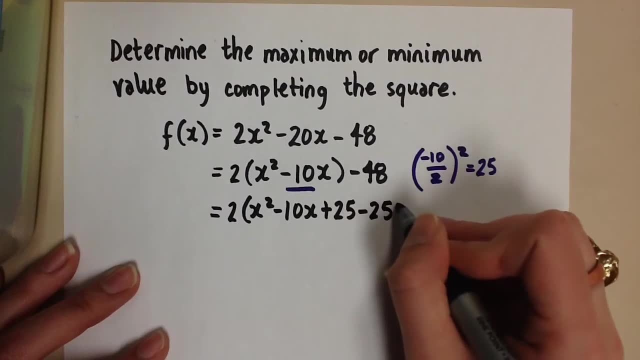 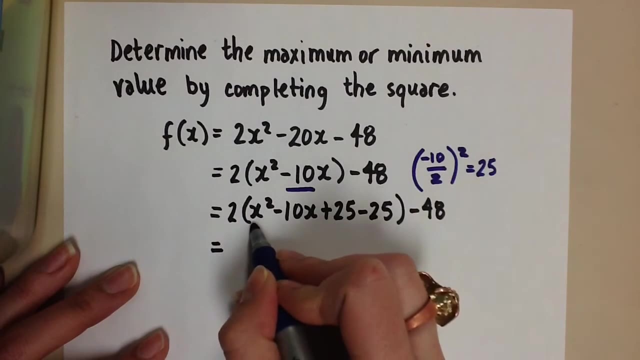 So we're going to go back to the equation here: x squared minus 10x. We're going to add 25 and then subtract the 25, and don't forget about the minus 48 outside of the brackets. So now we have this simple trinomial in the middle here. that is a perfect square.